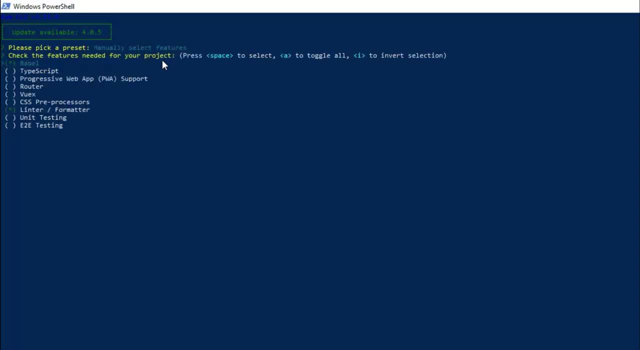 I can pick a preset. I want to manually select the features. I want to select Babel and I don't want to linter, So I will just click Babel here, because we are learning new concepts, we want to learn something new about components, So I'll just click here Babel. And where do you do? I prefer to? 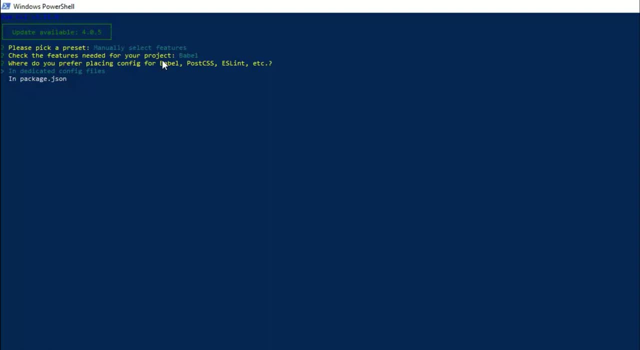 place a config file. So I will just say I want them to be in the dedicated config files. I don't want to save this preset and I will click No. So basically, right now we will. the new project is being installed, So I will just fast forward this, because we already 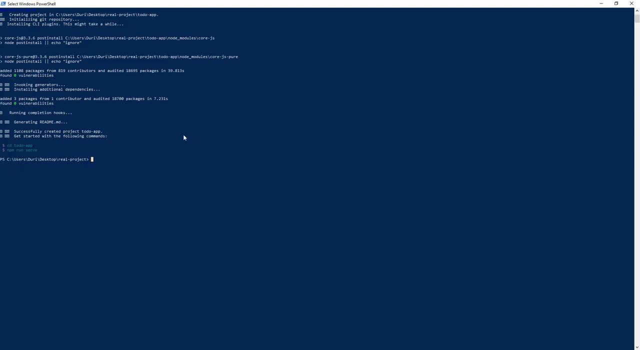 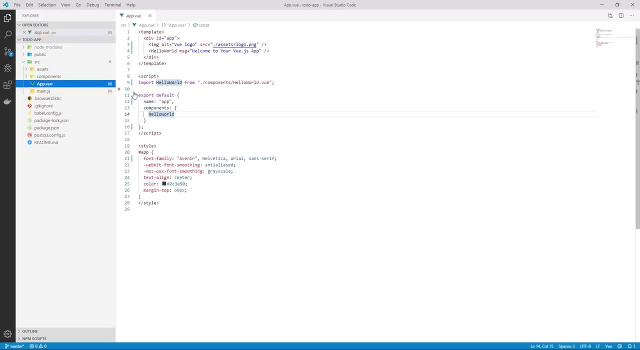 learned this. Okay, now, when the project is installed, I can actually open that project inside my IDE. And here's the project And, as you can see, here we have our app component. here is our main JS file And, as you can see, here the instance of the view application is created. 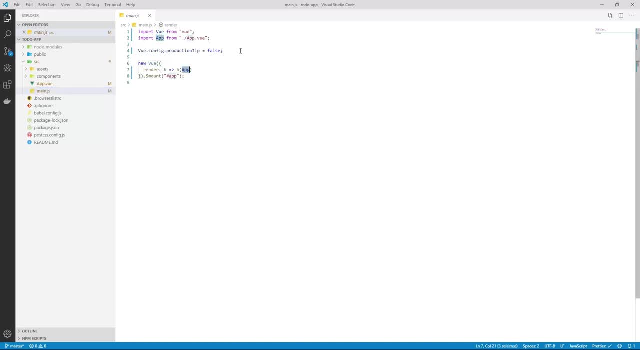 and then we are injecting this app component. So the app component is then being rendered as the first component, And we can see that the app component is being rendered as the first component. If we want to run this project, we will open the terminal and we will run npm, run serve And in a few 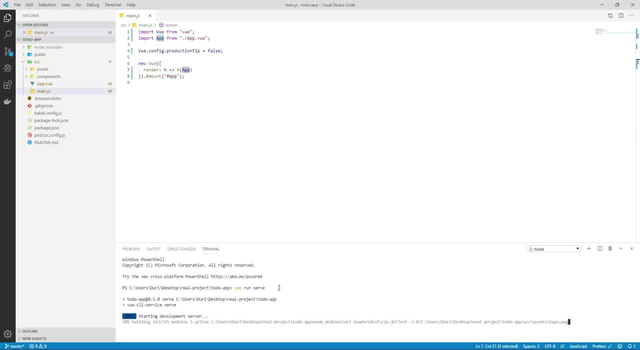 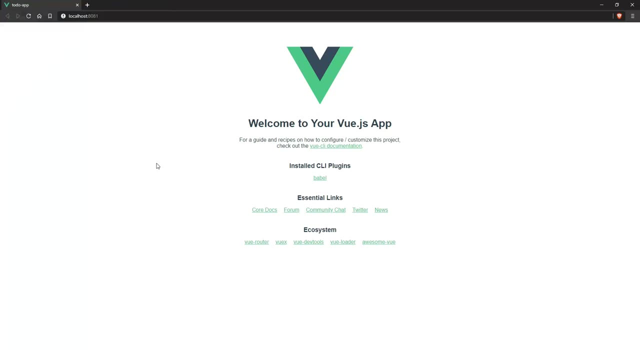 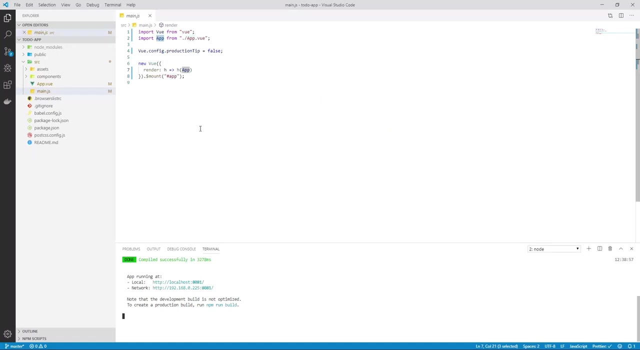 seconds. we will be then able to open our application. Exactly when I hit here, then here is our application. So the first aim is to actually create our first component. So let's try to create our first component, And in order to do that, 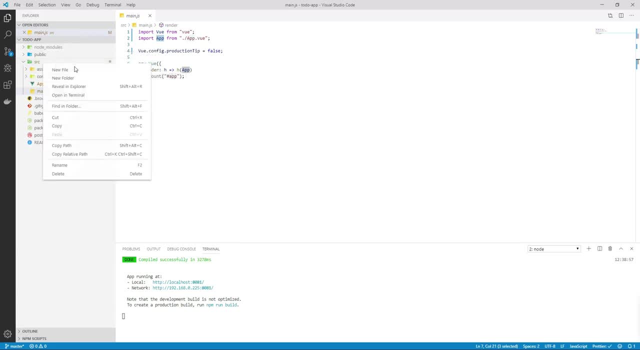 we will just click here on the source and create a new file, And the name of my new component is going to be my component component, dot, view. So the first thing to remember is the extension of this file is called view And I will explain briefly why we are doing that. So when I hit 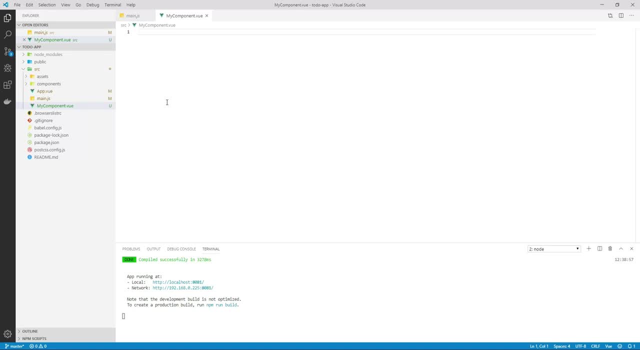 enter. this is now empty file And, as you can see here, my app component is being rendered as a IDE is recognizing that. this here, this file here, is a view component and that's why you see this view icon here. so this is our first component and let's try to implement it. so every component. 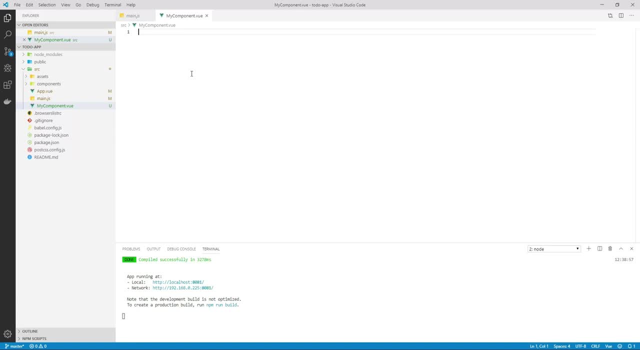 is a, let's say, the component is a building block of your view application. so everything you see on the website is going to be a component. so in order to create a component, you have to define, let's say, three different sections, and the first section is called a template section. 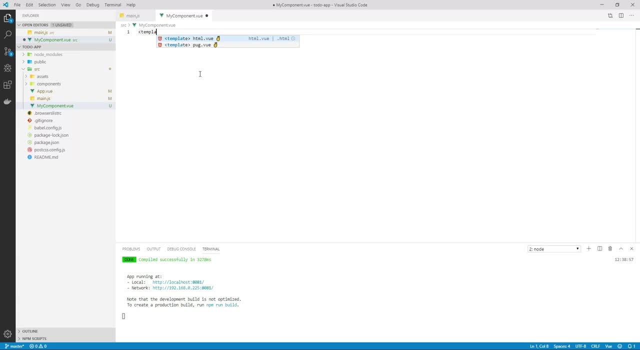 so when i start writing here, you can see that my id is suggesting me to click here, and then this template part is automatically rendered. i will, at the end of the video, i will explain you which plugin you have to use to create a component, and then you can see that. 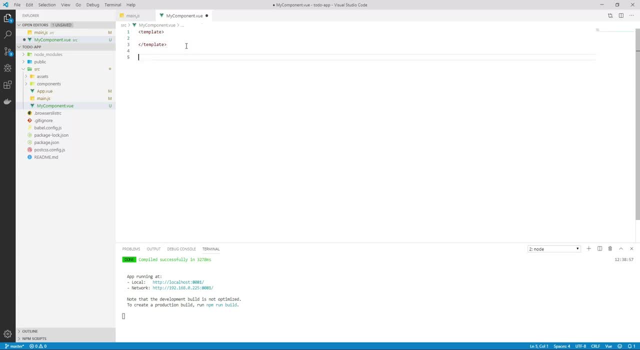 you have to install in order to have this. so the first thing of the component is a template. so inside the template you will write the html code that's going to be rendered inside the web browser. the second thing, or the second section of your component, is going to be: 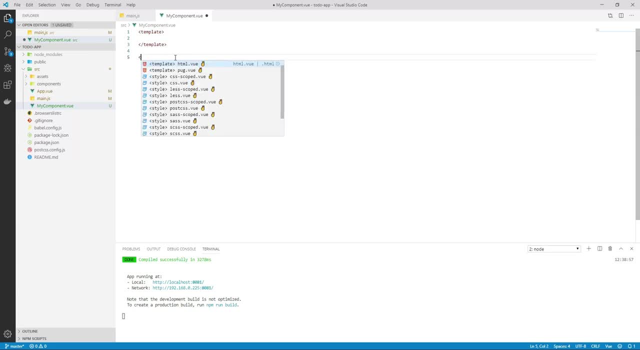 application logic or component logic, and this is a script, part of your application. and the third thing is the, the, the, the stylings or the css rules that are going to be applied for your application. and when, when you start writing style, then you will see here that the style, 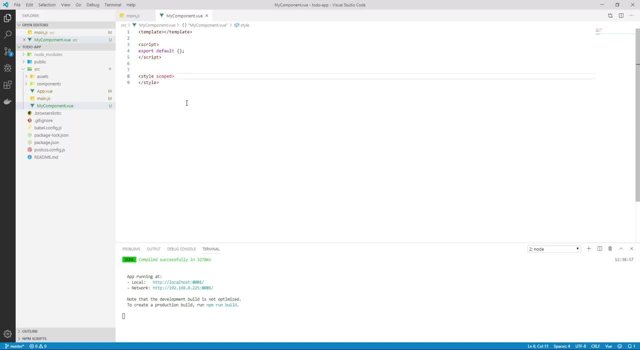 section is added and, believe it or not, this is exactly the thing: that you have to write these three things in order to create your first component. i want to note that if you, if your application, if your component doesn't have any logic, then you can also delete this part. 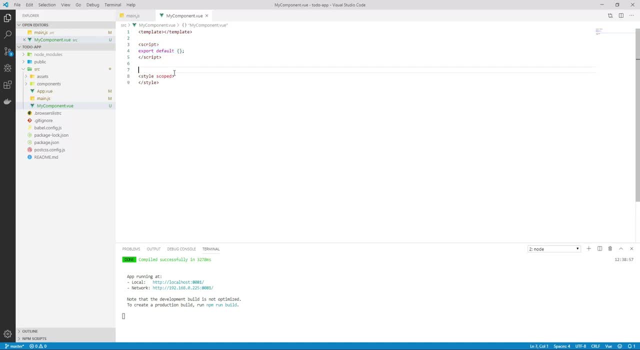 but for now, let's keep it like that. and here is the thing that i, when i mentioned that your component has needs to have this view extension, by doing that, you are able to write something like this. so by doing this, this is called single file component. so in this component, in this file, you are 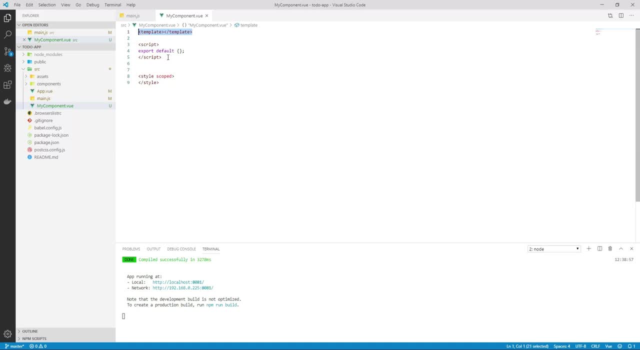 defining the design of your component. you are defining the logic- application logic or component logic- and you will also define here a css rules that are going to be defined for your component. so let's try to print something from our component. so i will add here a simple h1 tag. 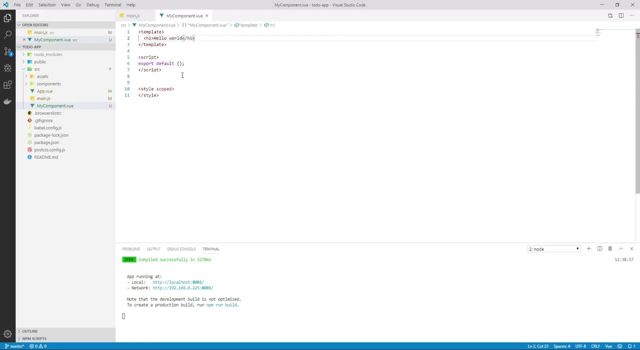 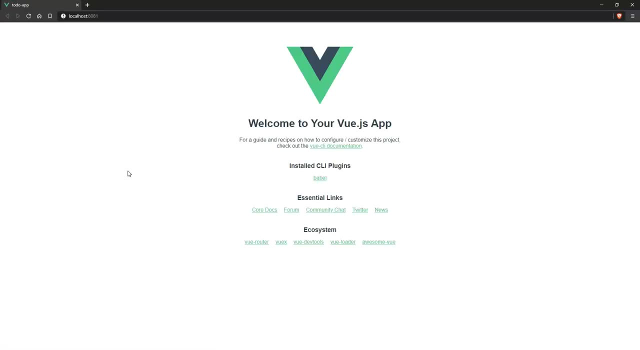 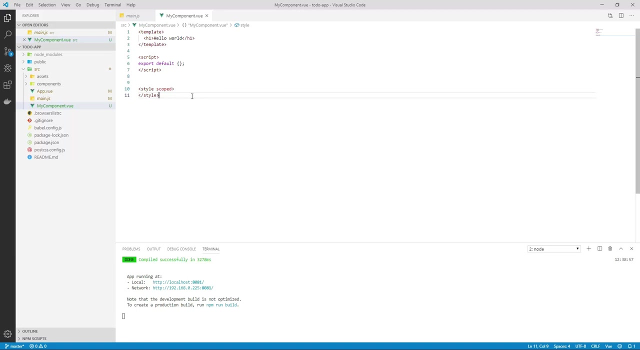 hello world and i will close this. and if i visit now, the web browser will show me that this is the web browser and if i refresh this page, you we will not see our component. well, that's happening because we never instructed the view framework to actually display our component. so, in order, 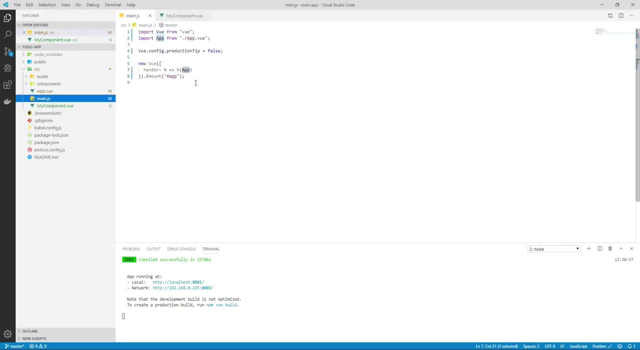 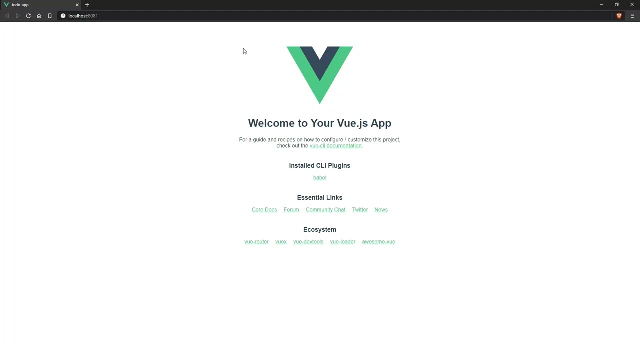 to do that, let's go to this mainjs file and, as you can see here, when the view application is starting, the first component we are injecting and the first first component that's going to be rendered is this app component, and that's why we are in the browser. we see this here instead of the text. that's. 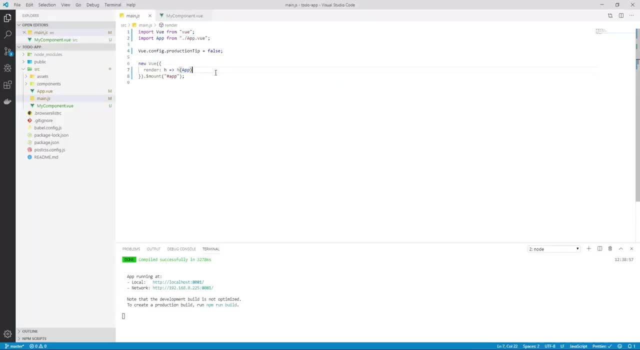 inside our component. so in order to do that, let's try to inject our component and not this app component, because my component is in the same level as an app component. i can write here my component dot view and here i can also write my component, and instead of injecting the app, 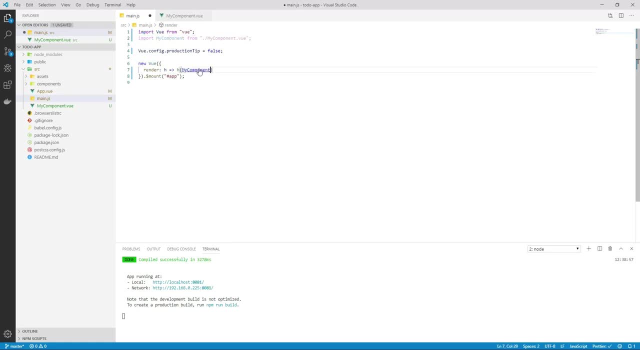 component. i can just inject my component, so i will just copy and paste this. so, right now, what's happening? when the view application is starting, the first component that's going to be rendered, is this, my component, or the component that we just implemented? so, if i go back now to the web browser, 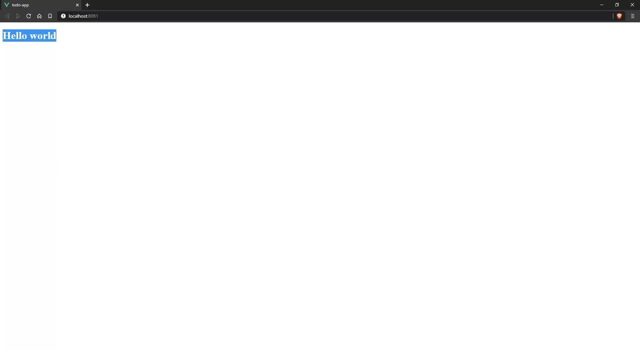 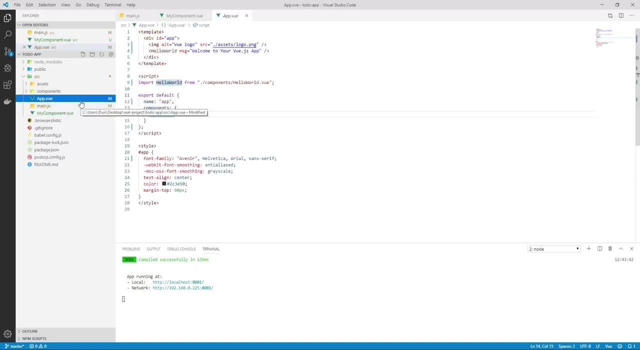 i will see this hello world text here. that's exactly the text that we printed inside my component, and what i want to do now is i want to delete this component. so i'm going to delete this appview component, because i don't need that component. i will work on my own component, so i'll 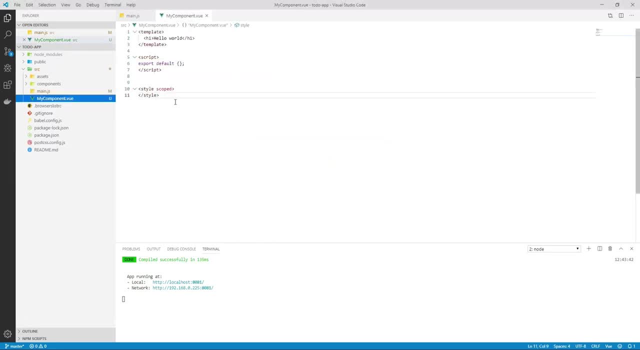 just delete this component. okay, so for now, everything is good, and the last thing that i want to mention here is, if you want to add a bit more text here, let's say i want to add h2 tag. this is our first component, and if i close this h2 tag, then you see here the component that we just 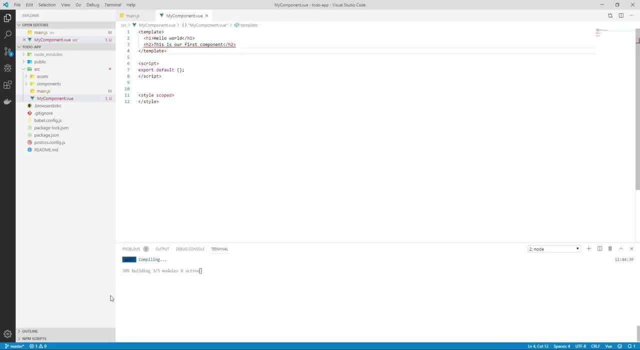 created and if i close this h2 tag then you will see here that there is some kind of an error here, and if i go back to the web browser, then you will see that application field to compile. so what's happening here? here is the thing you have to remember if you have multiple elements inside. 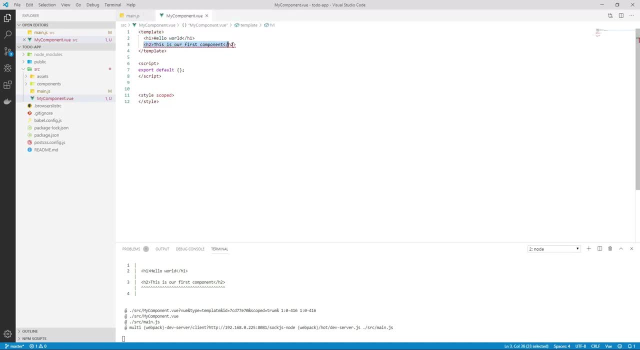 the template tag. so if, in my example, i have here h1 tag and then i have h2 tag, if you have these multiple elements, they have to be nested inside a single component. so if you have multiple elements inside a single root element, so what's that? so, in order to resolve this problem, let's define a div. 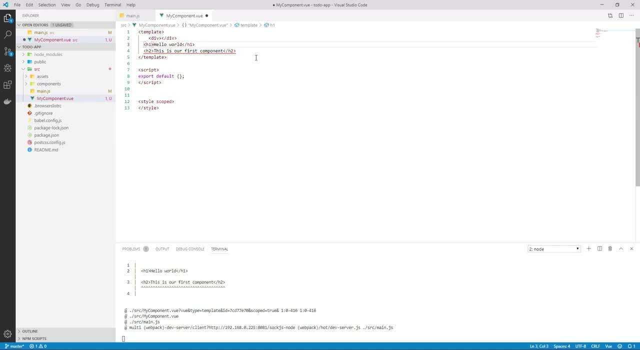 let's close this div and then let's put this content, these two elements, inside this div, and when i save this, what's happening here is i have a template, then i have a single root element, which is this div element, and following thatா, something about this div element. thank you for that´. 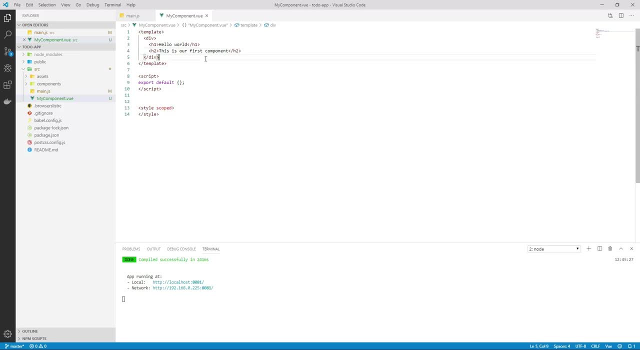 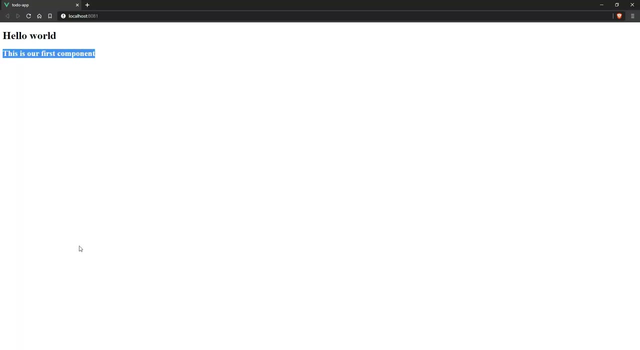 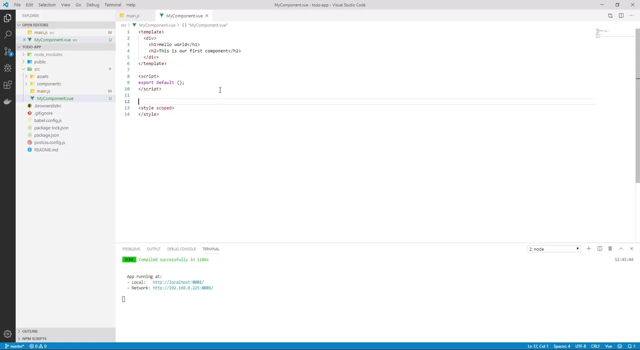 and this girl from excel, from certify, she says: if the first component does not exist, you must tell that, and i want to help me thatOK. so so it has just been a little nap. when I hit enters here a few times and when I save this component, this component is automatically. 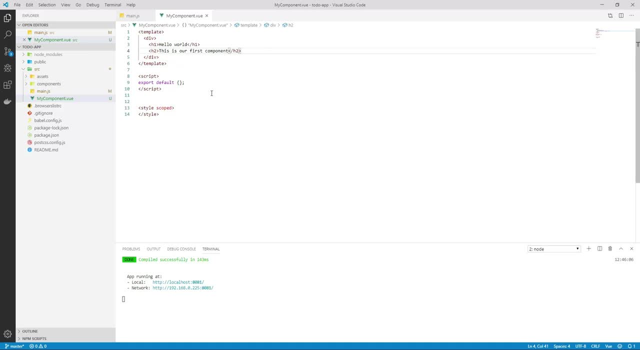 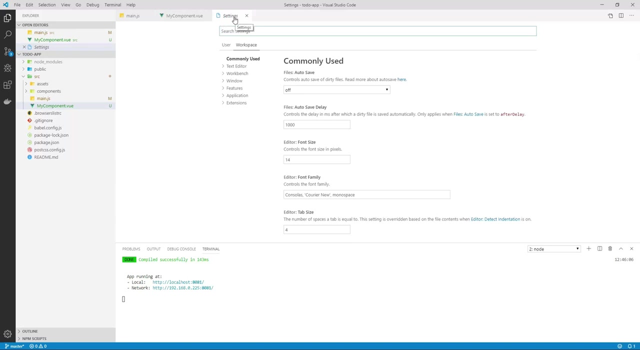 styled for me. so you can do that by clicking ctrl shift, p and here you can write workspace settings, and when you click here this window will open and then you can search something like format on save and click here on the user and just check this option here, format of, say, on save.